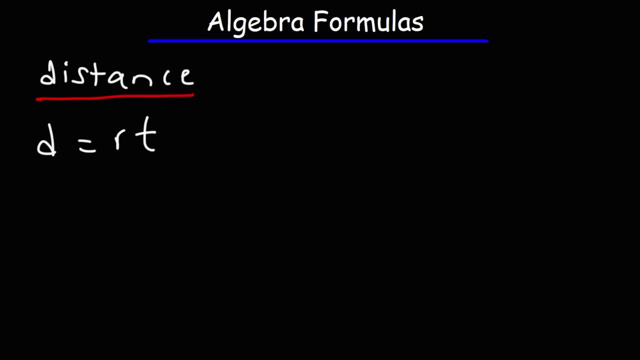 Distance is equal to rate multiplied by time. In physics it looks like this: d is equal to vt, Or displacement is equal to velocity multiplied by time. Now if you want to calculate the distance between two points, let's say you have point A and point B. 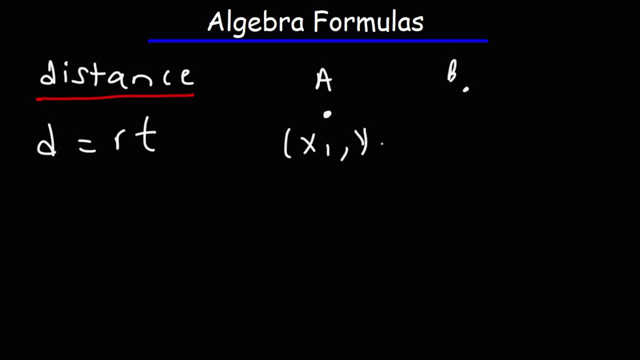 and you're given the coordinates of those two points, you can calculate the distance between the two points using this formula. So the distance is going to be the square root of x2 minus x1 squared, plus y2 minus y1 squared. Now let's say, if you want to find the midpoint between points A and B, 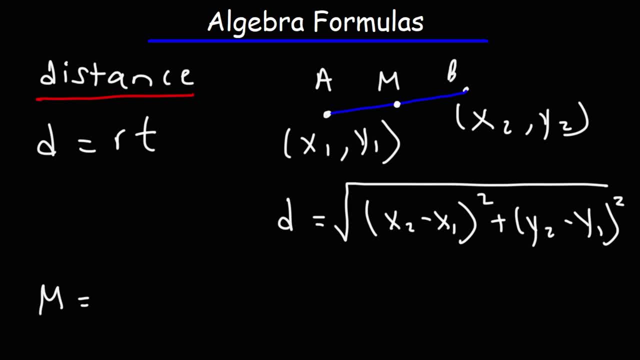 The midpoint. you could find that using the midpoint formula. The coordinates of the midpoint is going to be the average of the x-values and the average of the y-values. So that's how you can find the coordinates of the midpoint between points A and B. 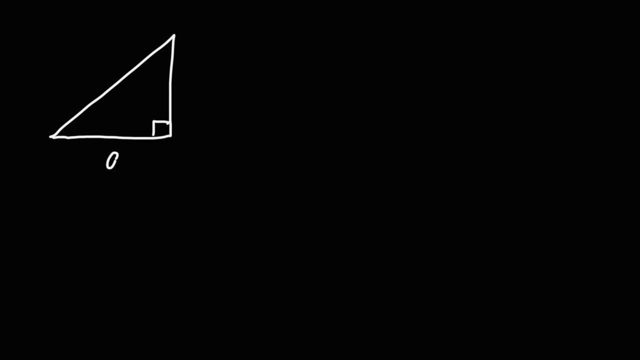 Now let's say we have a triangle where this is A, B and C. The next formula you need to be familiar with is the Pythagorean theorem. The hypotenuse C is equal to or C squared is equal to. 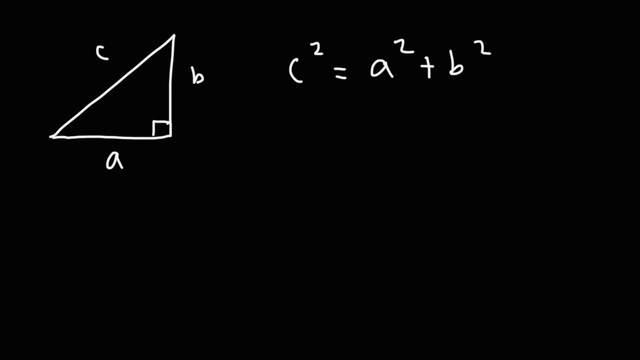 A squared plus B squared. Now, when dealing with triangles, you need to be able to calculate the area of a triangle. The area of a triangle is 1 half base times height. When dealing with circles, the area is pi r squared. 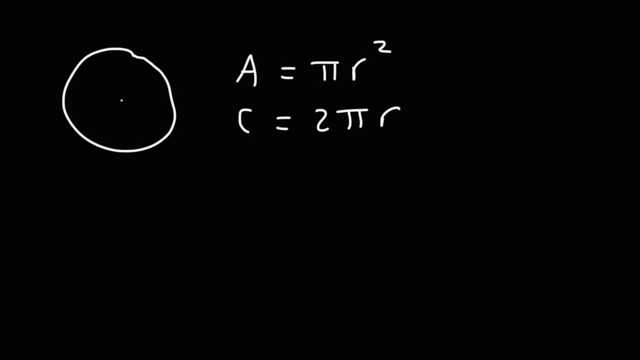 The circumference is 2 pi r. The radius is the distance between the center of the circle and any point on a circle. The diameter is twice the value of the radius. Now the equation of a circle is this: x minus h squared, plus y minus k squared, is equal to r squared. 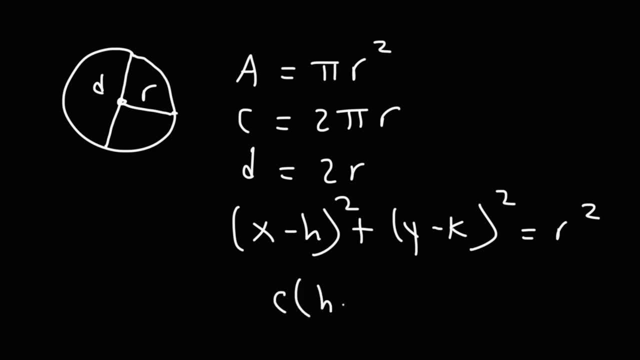 In that standard form, the center of the circle has the coordinates h, comma, k and r is the radius: The radius of the circle. Next we have a rectangle with a length and a width. The perimeter of the rectangle is 2l plus 2w. 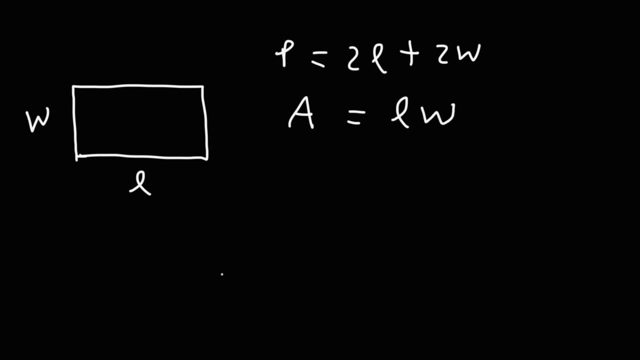 The area of the rectangle is length times width. For squares with side s, the area of a square is s squared. The perimeter is 4s. The perimeter is the distance around the object. Now, the next thing we're going to talk about is the simple interest formula. 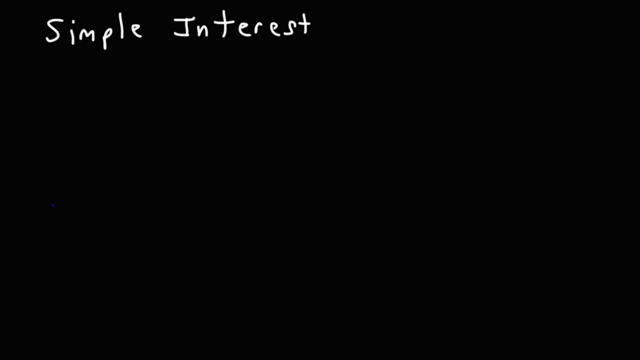 There's simple interest and there's compound interest. The simple interest is equal to the principal times, the annual interest times, the time in years. Now for compound interest. here's the formula: The future amount or the future value is equal to the principal times e raised to the interest rate times t. 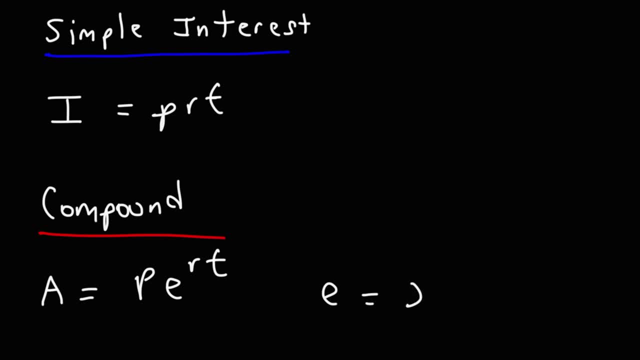 And t is in years as well. e is a special number, It's 2.71828, and some other numbers after that. To find the exact value of e, you could use a calculator And just type in inverse natural log. It'll give you the exact value of e, which is 2.718281828.. 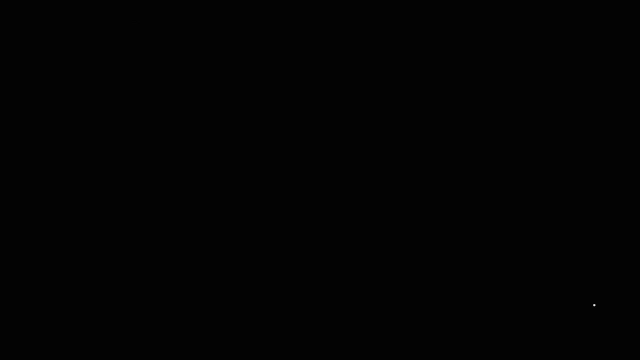 And it repeats. Now let's talk about linear equations. This is a very common topic in algebra, So there's three forms in which you can write Linear equation. The first one is standard form. Ax plus By is equal to C. 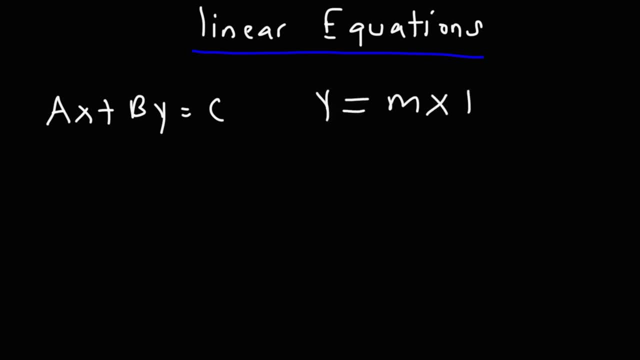 The next one is its slope-intercept form. Y is equal to Mx plus B. M represents the slope, B represents the y-intercept. And then there's the point-slope formula: Y minus Y1 is equal to M times x minus x1.. 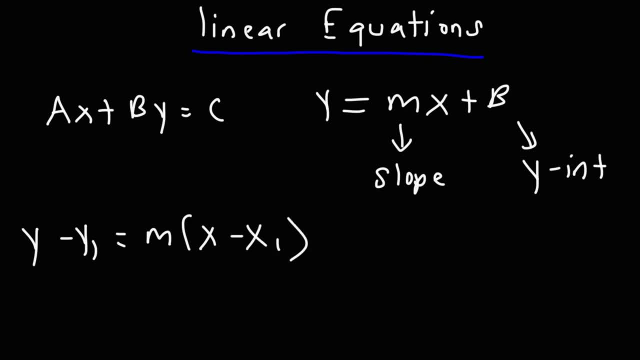 So those are the three common equations that you'll use if you want to write linear equations. Now, to calculate the slope between two points, it's the change in y, y2 minus y1 divided by the change in x, So it's rise over run. 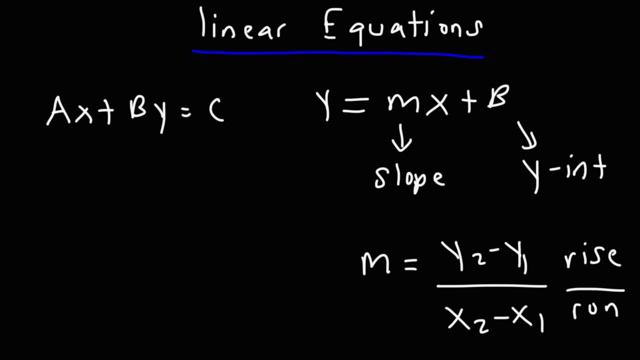 The slope formula is very similar to the average rate of change formula. To calculate the average rate of change, it's the change in y or f of x2 minus f of x1, divided by the change in x. The average rate of change formula is the same as the slope formula. 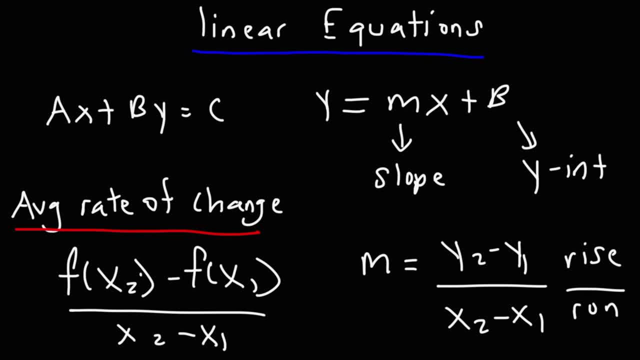 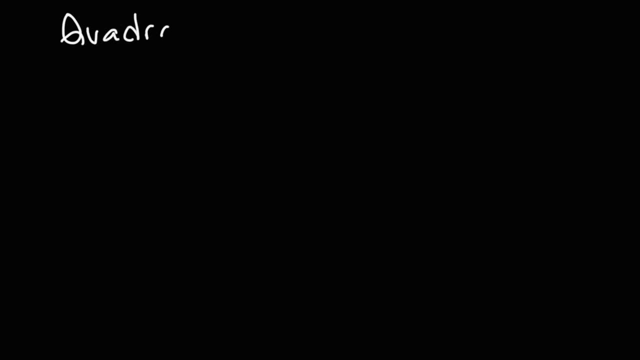 The average rate of change gives you the slope of the secant line. A secant line is a line that touches two points on a curve. A tangent line only touches one point on a curve. So that's the slope formula. Now let's move on to the formulas associated with quadratic equations. 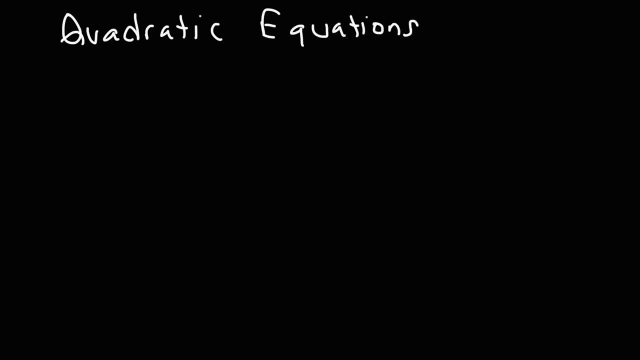 Let's say you have a quadratic equation in standard form and it's set to zero. So we have ax squared plus bx plus c is equal to zero. If we want to calculate the value of x, We could use the quadratic formula. It's negative b plus or minus the square root of b squared minus 4ac, all divided by 2a. 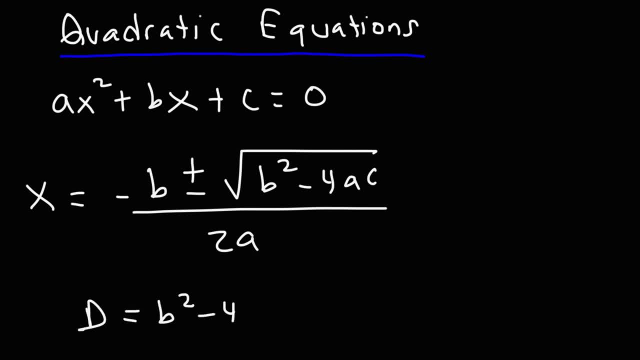 The discriminant is b squared minus 4ac. It's the stuff inside of the square root. If the discriminant is positive, if it's greater than 0, that means you have two real solutions. If it's equal to 0, you have one real solution. 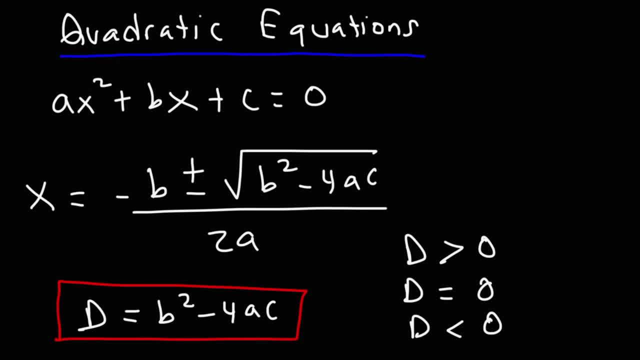 If it's less than 0, or if it's negative. that means you have two imaginary solutions. The imaginary number i is equal to the square root of negative 1.. So anytime you get a negative value inside of a square root, you're dealing with imaginary numbers. 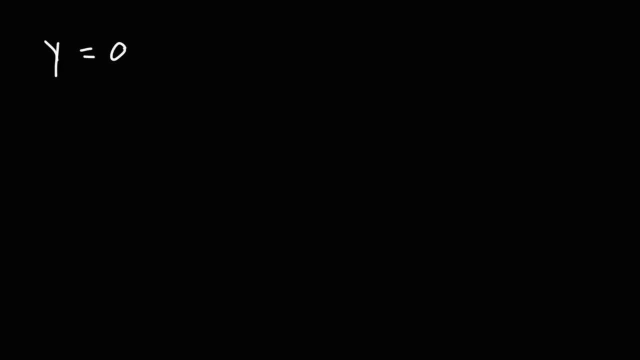 Now sometimes you might have a quadratic equation written in vertex form. So y is equal to a a times x minus h, squared plus k. In vertex form the coordinates of the vertex of the parabola is h comma k. So let's say you have a graph that looks like this: 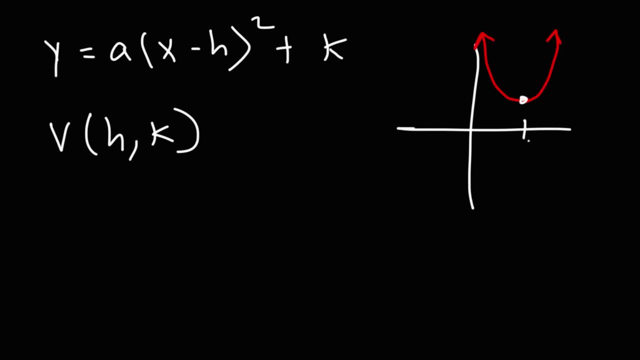 This is the parabola. Here's the vertex. This is h, This is k. This is also the axis of symmetry. You could find the axis of symmetry Using this formula. It's negative b over 2a, But this works if the quadratic equation is in standard form. 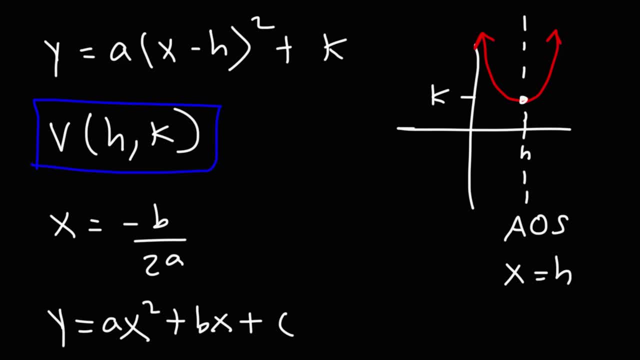 If it's in vertex form, the axis of symmetry is simply going to be: x equals h, So you just got to look at whatever this number is. If it's in standard form, then use this formula to get the axis of symmetry. Now let's talk about formulas associated with factoring. 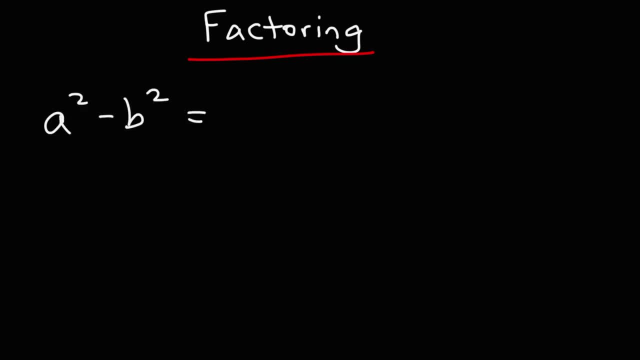 So let's say you have a difference of two squares, a squared minus b squared. To factor it, it's going to be a plus b times a minus b. Now let's say you have a difference of two cubes: a cubed minus b cubed. 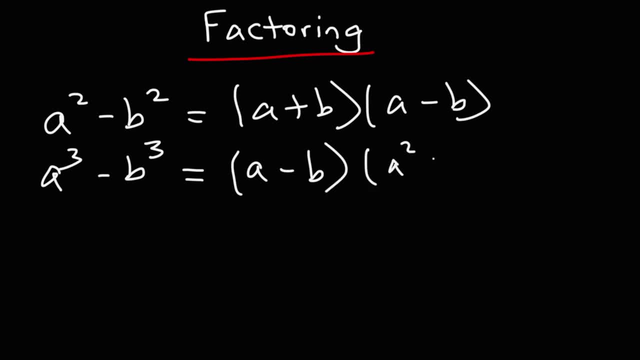 To factor it, it's going to be a minus b times a squared, plus a, b plus b squared. If you have the sum Of two cubes instead of a minus b, it's going to be a plus b, and then it's going to be a squared. 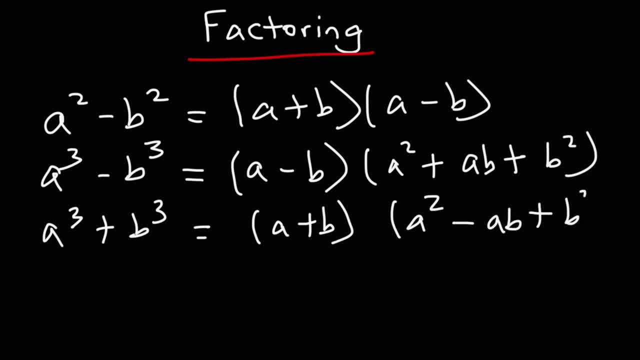 But instead of plus a b, it's minus a, b and then plus b squared. Now if you have a perfect square trinomial- a squared plus two, a, b plus b squared- to factor it, it's simply going to be a plus b squared. 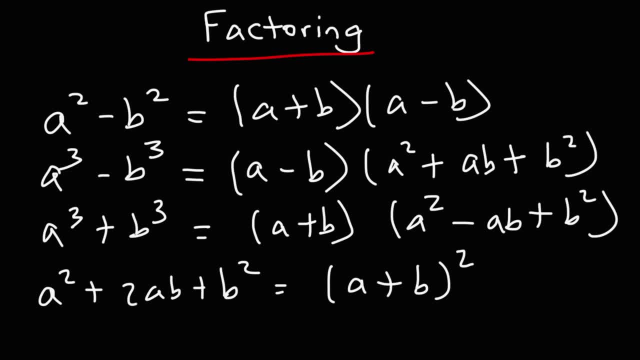 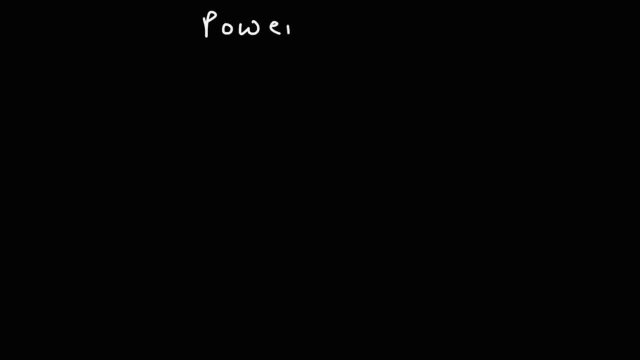 So those are some formulas to know when you're factoring algebraic expressions. Now the next thing we need to talk about are powers and exponents, particularly the rules associated with these. So first, multiplication: If you multiply two variables, the variables are the same kind but with different exponents. you need to add the exponents. 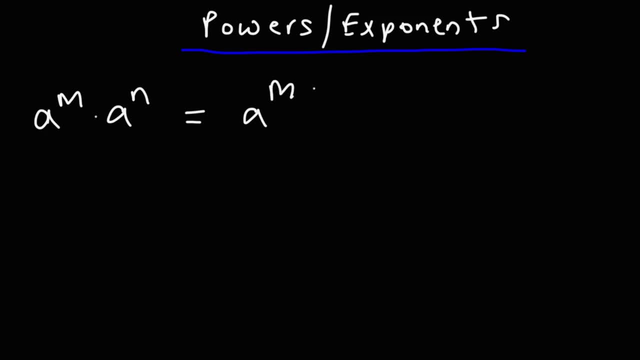 So a to the m times a to the n is a to the m plus n. So, for instance, x to the third times x to the fourth, that's going to be x to the three plus four, which is x to the seventh. 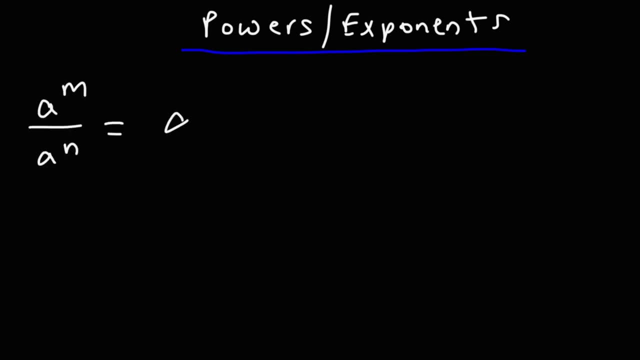 When you're dividing variables you need to subtract the exponents. So this is going to be a to the m minus n. So if we have x to the nine divided by x to the four, this is going to be x to the nine minus four, which is x to the five. 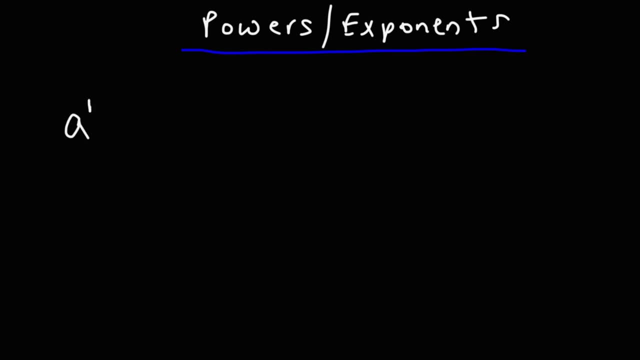 Now, when you raise an exponent to another exponent, you need to multiply the two exponents, So x to the third raised to the sixth power, this is going to be x to the third times six, or three times six, so that's x to the eighteenth. 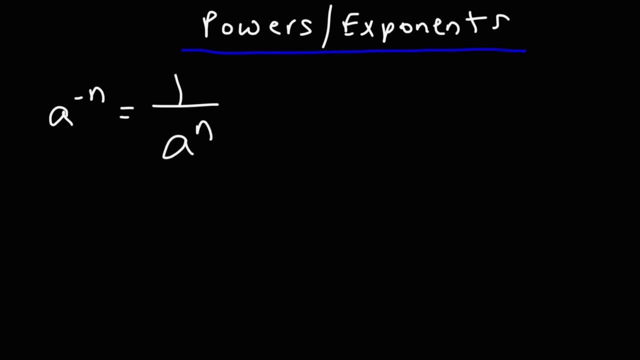 If you have a negative exponent you can make it positive by moving the variable to the bottom. So x to the negative, four Is one over x to the four And one over x to the negative, five is x to the five. So whenever you move the variable from the top to the bottom, it's going to change. sign: 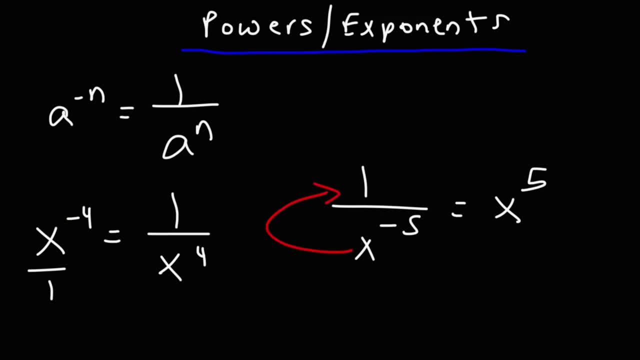 Or if you move it from the bottom to the top, it will also change. sign Now: anything raised to the zero power is one. So if you have x squared y to the third, raised to the zero power, that's going to equal one. 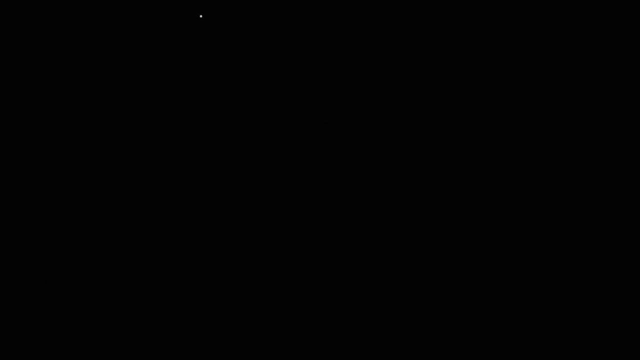 Now let's move on to the property of logarithms. Log a raised to the x. you can move the x to the front. This is equivalent to x times log a. Log ab. you could separate that into the sum of two logs. 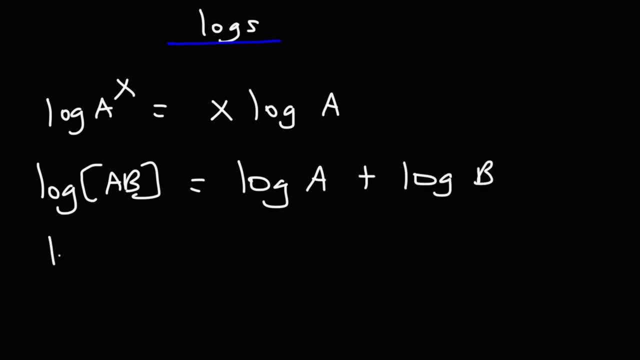 It's log a, Log a plus log b, Log a over b. you could break that into the difference of two logs. It's log a minus log b. Now the next formula we need to talk about is the change of base formula. 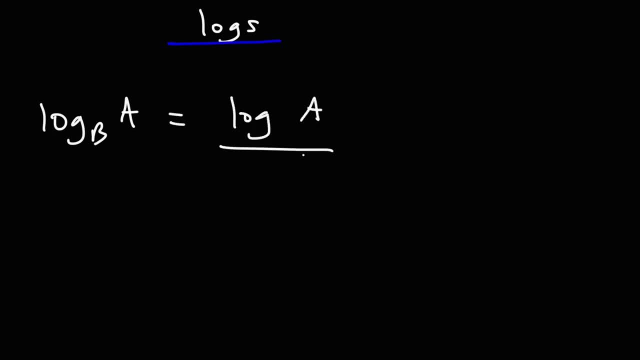 Log b of a. this is equal to log a over log b. Log b And there's going to be a new base c. That could be any number. It could be 7,, it could be 5,, it could be 12.. 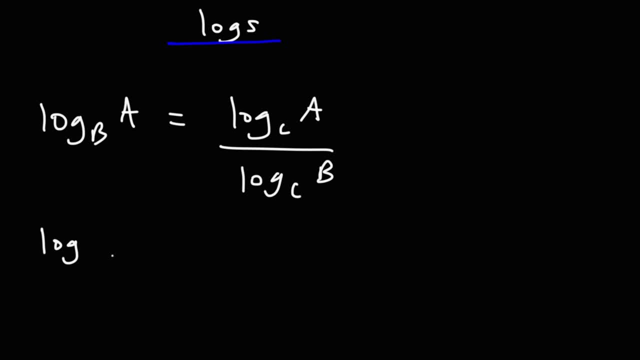 It doesn't matter what number you choose, it will be the same. So, for instance, let's say we have log 5 of 9. This is going to be log 9 over log 5. The new base. I can make it anything. 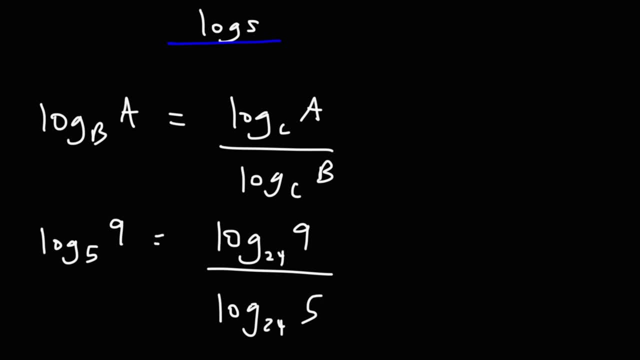 I can make it 24 if I want to, And it will still be accurate. So that's the change of base formula. As we can see, the base was changed. The base was changed from 5 to 24.. Now let's talk about variation. 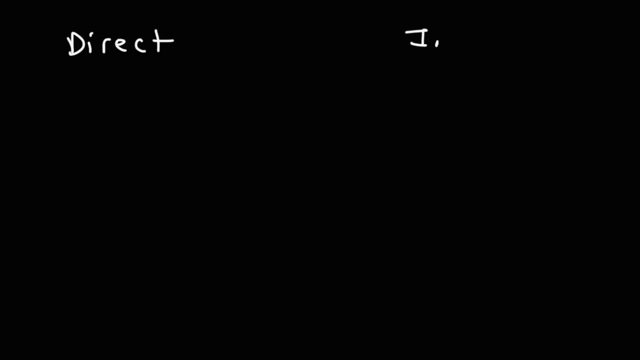 There's direct variation and then there's inverse variation, And let's talk about the formulas associated with this. So for direct variation, we have the formula y is equal to kx. For inverse variation, it's y is equal to k over x. 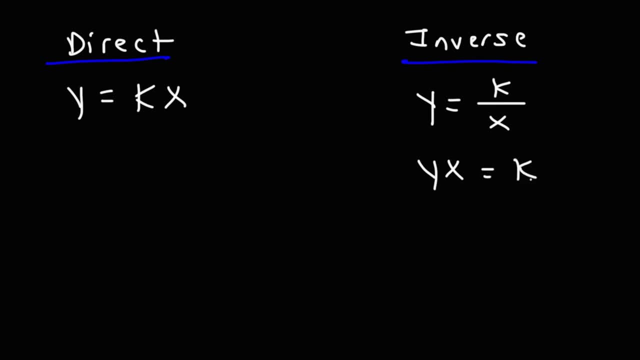 You could also write this as: y times kx. Y times x is equal to k. k is the constant of variation. In direct variation, when x goes up, y goes up. For inverse variation, when x goes up, y goes down. 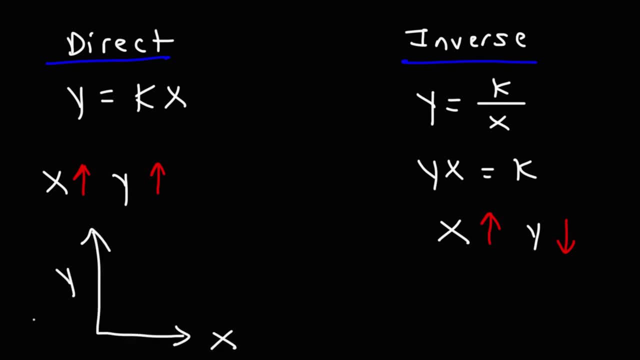 So for direct variation, you have a graph that looks like this: It's a linear relationship. For inverse variation, where y is equal to k over x, it looks like that. Now let's talk about arithmetic and geometric sequences. Let's go over some formulas for these two concepts. 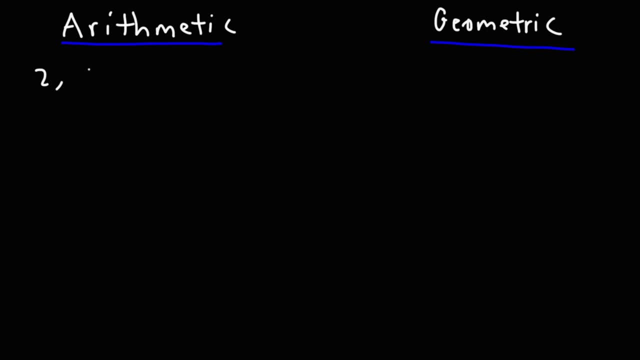 Now, when you have an arithmetic sequence, the numbers increase by a constant amount. So in this case the common difference is 3. The numbers are increasing by 3. You have to add 3 to get to the next number. For a geometric sequence it's different. 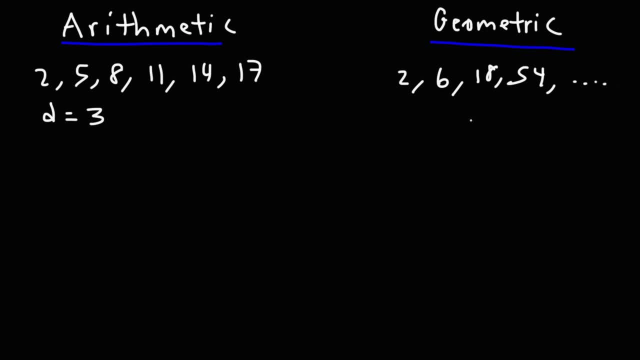 Notice that to get the next number you need to multiply by 3. So you get a common ratio called r. So r is 3. in that case a1 is the first term, So here a1 is 2.. a2 is 5.. 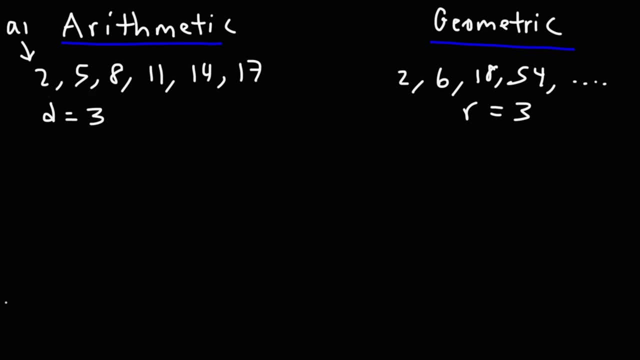 a3 is 8.. a4 is 11.. To find the nth term, it's equal to the first term plus n minus 1 times the common difference For geometric sequence. to find the nth term: it's equal to the first term times the common ratio raised to the n minus 1.. 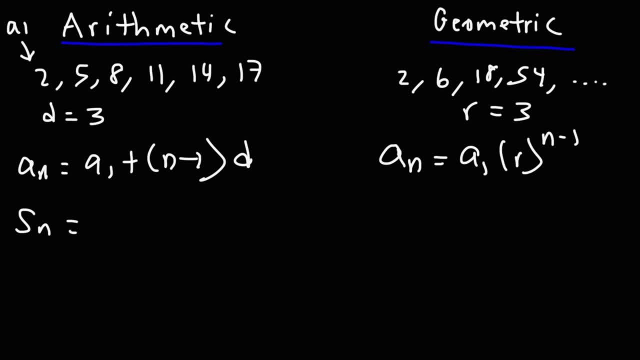 Now, if you want to find the sum of a certain set of terms, it's going to be the first term plus the last term, And then it's divided by 2 times the number of terms. For geometric sequence, it's going to be the first term times 1 minus r raised to the n over 1 minus r. 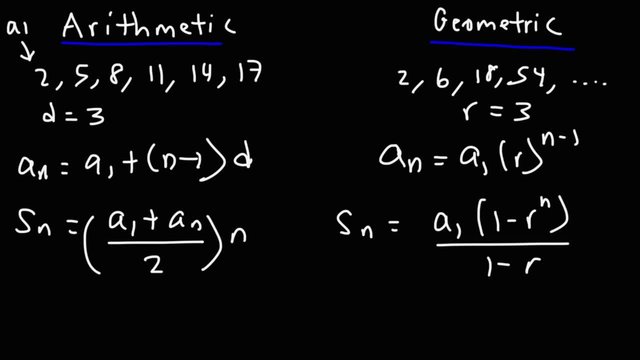 Now, if you have an infinite geometric sequence, particularly when r is less than 1, you can calculate the sum of an infinite geometric sequence using this formula. Basically, you just get rid of this part, But this only works if you have an infinite geometric sequence. 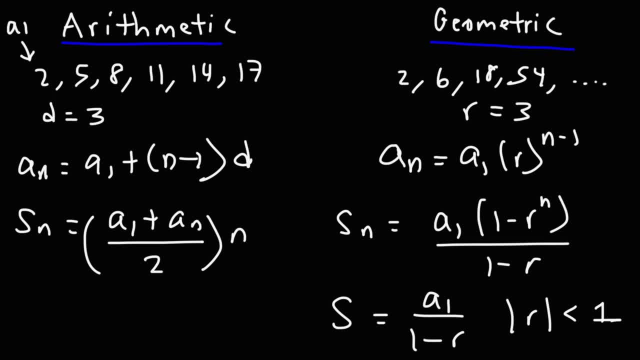 So you can calculate the sum of an infinite geometric sequence using this formula. Basically, you just get rid of this part, But this only works if the absolute value of r is less than 1.. So instead of the numbers increasing, they should be decreasing when r is less than 1.. 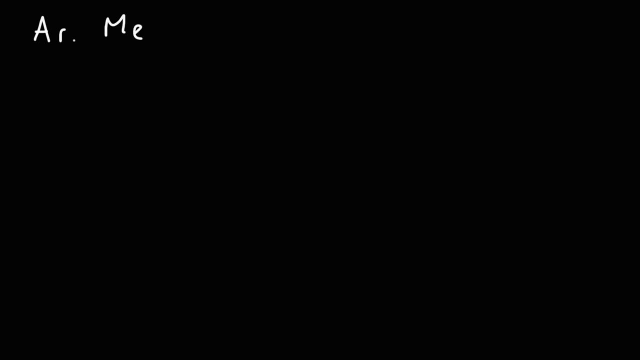 Now to calculate the arithmetic mean. there's a difference between the arithmetic mean and the geometric mean. The arithmetic mean of two numbers is simply the absolute value of r. The arithmetic mean of two numbers is simply the absolute value of r. The arithmetic mean of two numbers is simply the absolute value of r. 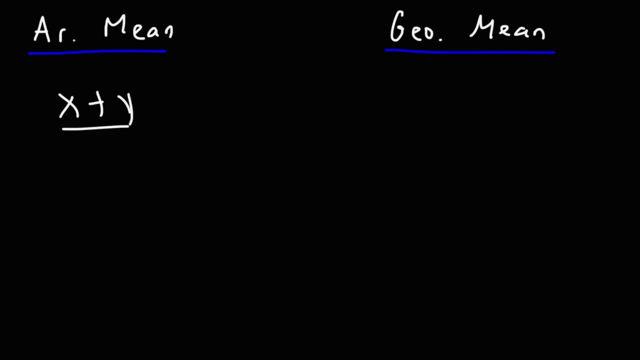 The average of those two numbers is the sum of the two numbers divided by 2.. The geometric mean of two numbers is the multiplication of the two numbers And instead of dividing it by 2, you need to take the square root, which has an index of 2.. 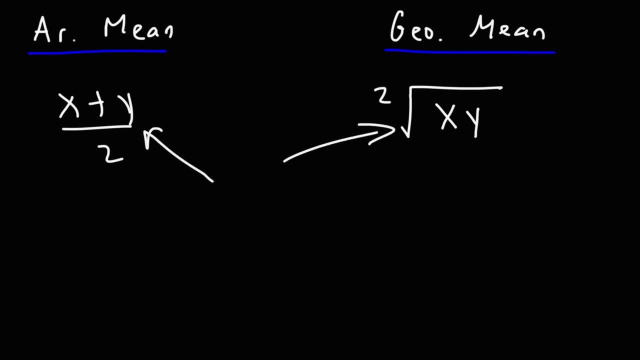 So this is how you calculate the arithmetic mean and that's how you calculate the geometric mean. Now, going back to our previous example, where we had this particular arithmetic sequence, if we calculate the arithmetic mean of these two numbers, it will give us the middle number. 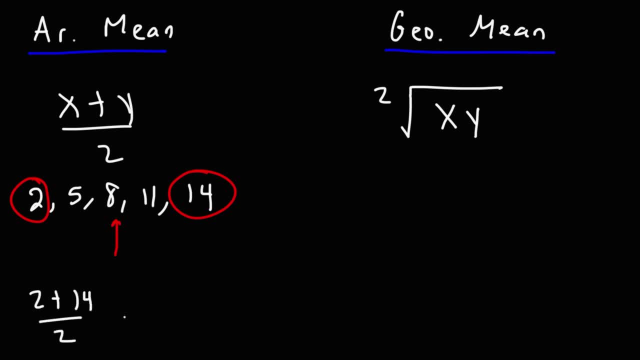 So 2 plus 14 divided by 2.. 2 plus 14 is 16, divided by 2 is 8.. Now if we were to extend this, and let's say we want to find the arithmetic mean of 2 and 20,, 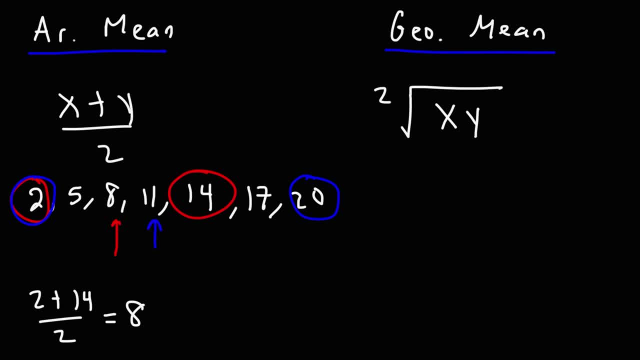 it'll give us the middle number. 2 plus 20 is 22.. 22 divided by 2 is 11.. Now for a geometric mean. it works the same way. So let's say we have the numbers 2,, 6,, 18,, 54,. 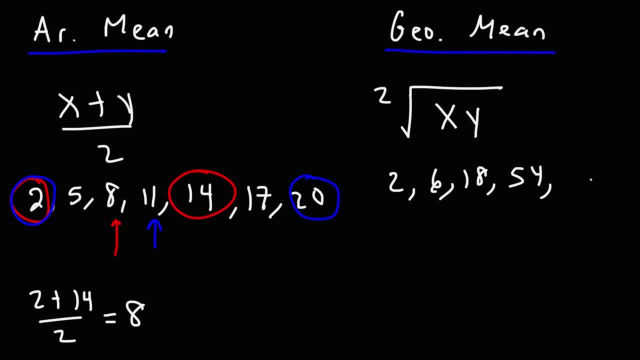 and then 54 times 3, that's 162.. So let's say we want to find the geometric mean of 2 and 162. It will give us the middle number 18.. So if we take the square root of 2 times 162,, 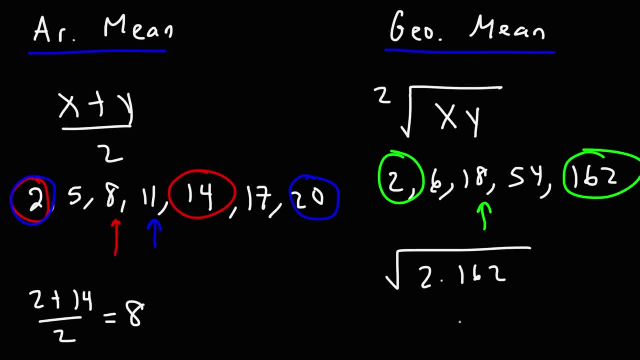 2 times 162 is 324.. And the square root of 324 is 18.. So the arithmetic mean gives you the middle number of the two numbers in which you were looking for the arithmetic mean of Same thing for the geometric mean. 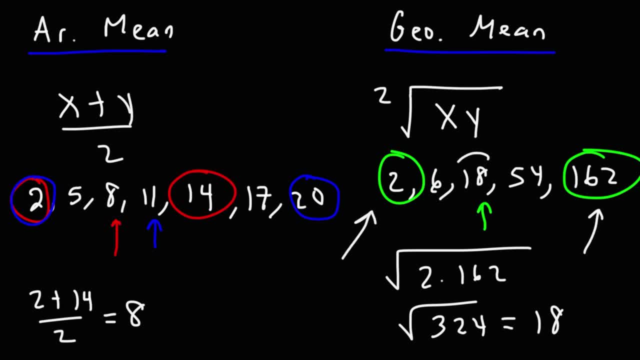 The geometric mean of two numbers will give you the middle number in a geometric sequence. 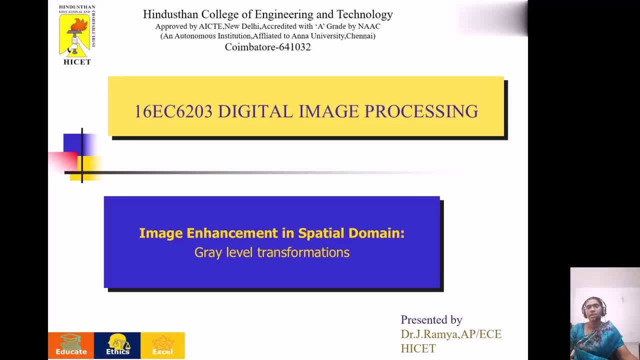 Good morning all. Myself Ramya, working as Assistant Professor Department of EC at Hindustan College of Engineering and Technology, Coimbatore. I am here to discuss about image enhancement in spatial domain under that grey level transformations which comes under the subject of digital image processing. 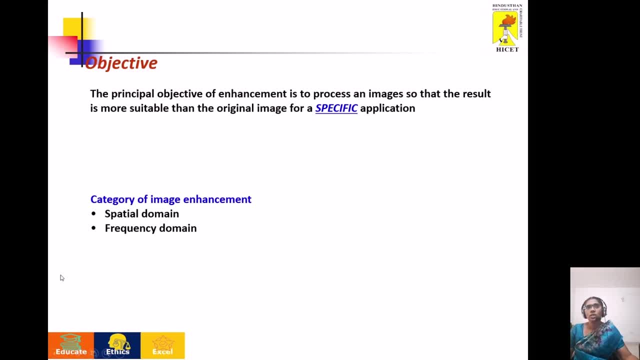 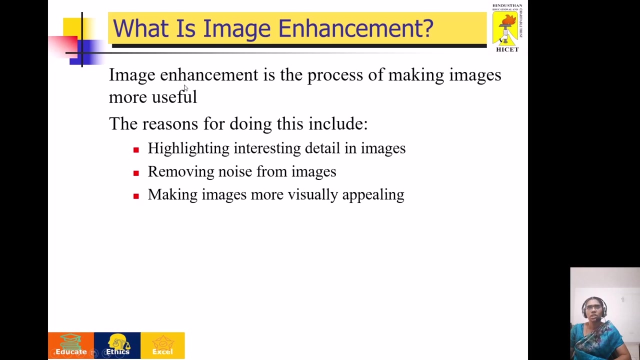 So image enhancements main purpose and main objective is to make the image which is more suitable than the original image. So it has to be made better for visual perception and this algorithm may differ according to the application. The image enhancement can be spatial domain or frequency domain. And what is image enhancement? The image enhancement is the process of making the images more useful. 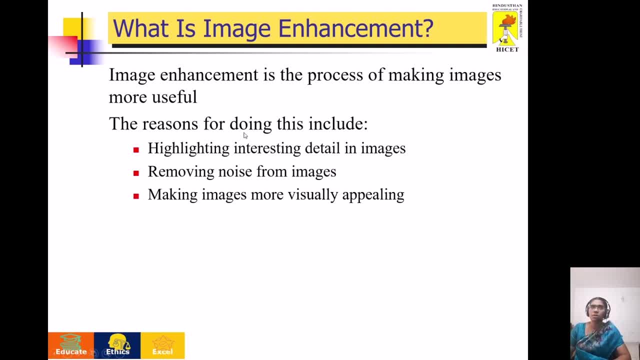 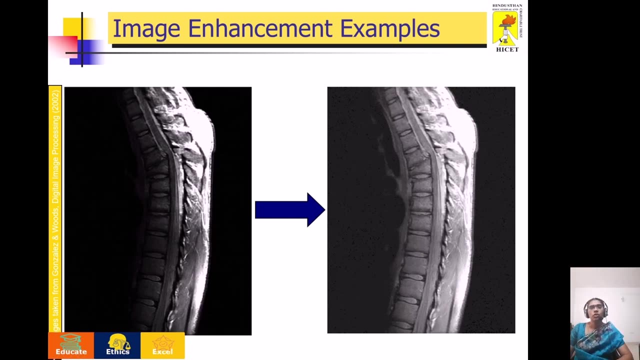 And the second necessity in this, very quickly, all of the aspects we are going to discuss about image enhancement is the quality of the image. So now the aspects of image enhancement are: notование the spines of the X. is that the image that appears in a form by using up, so in this case it is the animal doll.